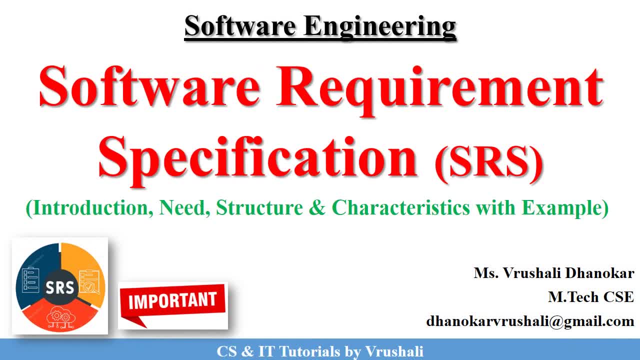 Hello everyone, this is Vrishali. In previous sessions we discuss about all SDLC models and requirement engineering process with example. I have mentioned complete software engineering subject playlist link in below description box. Now in today's session we will discuss about the next important topic, that is, software requirement specification, or SRS document. 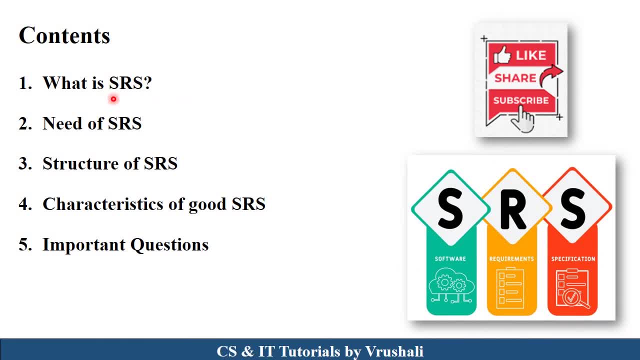 Let's start the session. In today's session we will discuss about what is SRS, their need, their structure, characteristics of good SRS and some important questions that have asked in previous year question paper. Now let's see all these points one by one. The first: 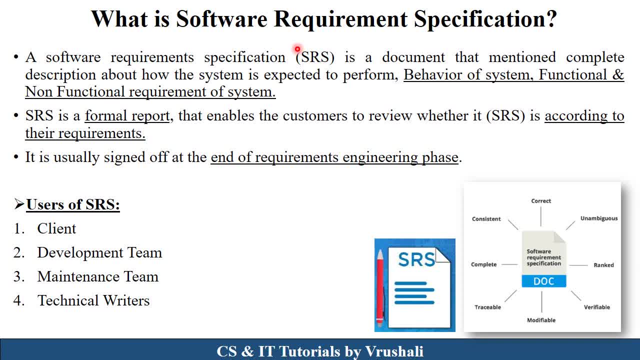 thing is what exactly SRS See. as we discussed earlier, in software development life cycle, the first phase is requirement gathering and analysis phase. Here, project head collect all the requirements for SRS From the customer. Now this, all requirements, are mentioned in one document, This document. 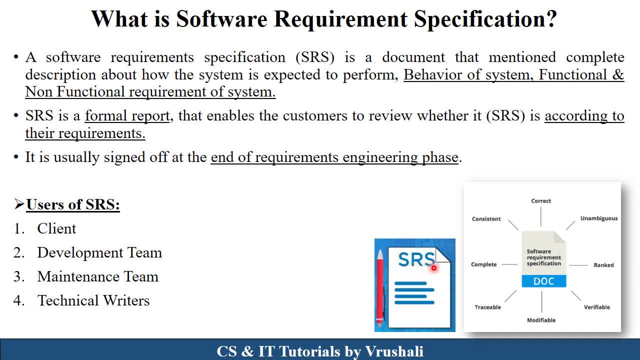 is called as SRS, that is, software requirement specification document. As per the definition, SRS document mention complete description about how the system is expected to perform, behavior of system and functional and non-functional requirement of system. They mention every requirement discussed with the customer. Basically, SRS is a formal report. 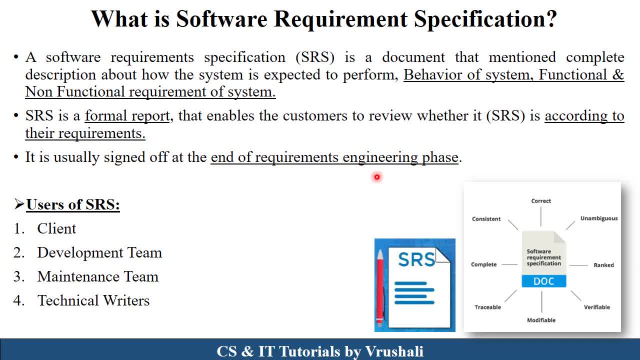 And this report sign off at the end of requirement engineering phases. These are the different users of SRS, like client and customer use the SRS document to check that, whether every requirement have mentioned clearly or not. Development team use for development purpose and maintenance team. technical writers use the SRS document as per their requirement. 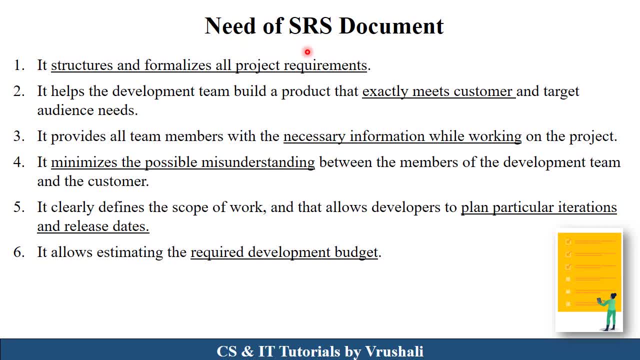 Next. the next thing is need of SRS document. Why SRS document have generated at the end of requirement gathering phase? First, SRS document: mention every requirement discussed with customer in proper structure manner. Second thing is developer: use SRS document for development purpose because it 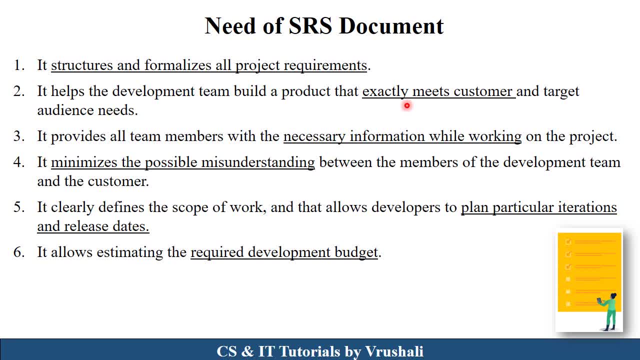 check that every requirement have exactly meet with the customer. SRS document also provide all the necessary information to all the team members. For example, developer use SRS document for development purpose to check the requirements. then tester use SRS document for operation. Next, development team use SRS document for program's development. 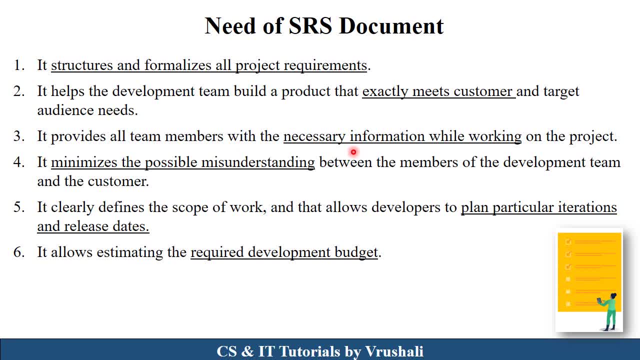 test cases purpose basically provide all the necessary information to all the team members. it also minimize misunderstanding between development team and the customer because every requirement have mentioned simple and clear manner. due to SRS document, developer decide the delivery date or final release date of the particular product. and due to SRS document. 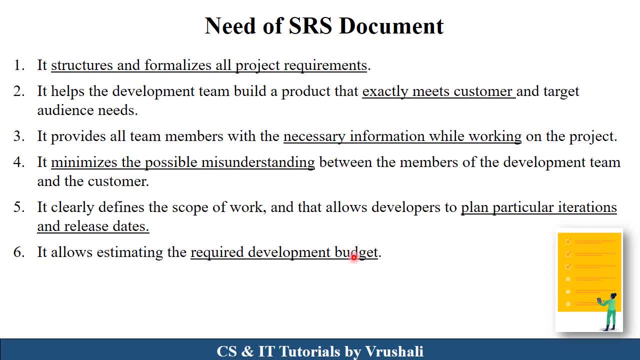 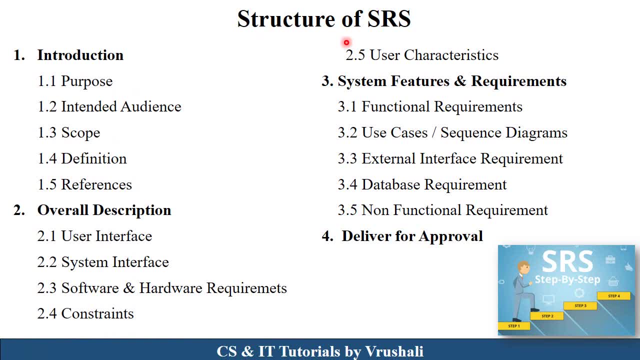 everything mentioned clearly so it easy to find out overall budget of the project. so these are the need of the SRS document. the next thing is structure of SRS, how to rise SRS document. so let's take the example of college management system. the first part of SRS document is introduction. here you have 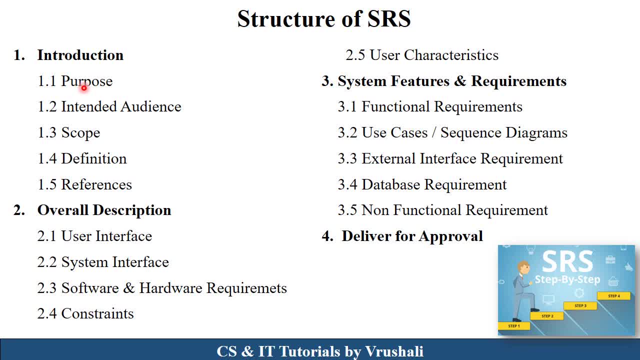 to mention the purpose behind developing college management system. application means which type of organization used the particular product, the aim, the goal behind developing a particular project. next one is the intended audience minutes means which type of user use the particular application, for example, the college management system application used by student teachers, hod principals. so these all are the intended audience. 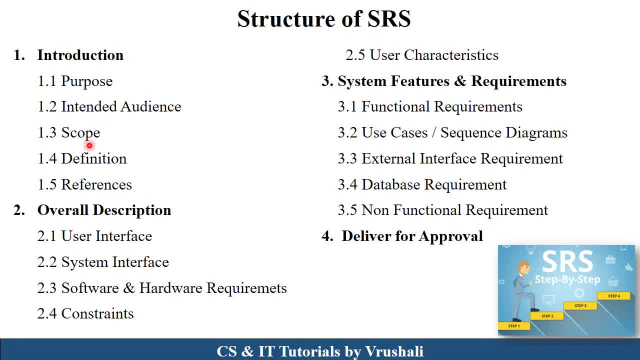 next one is a scope. scope means future of particular project. in future you can add some additional features and also college management system application used by universities also. so what will be the future of particular project here? you have to mention it. next one is the definition. we can say definition means some abbreviations or some short forms, for example: 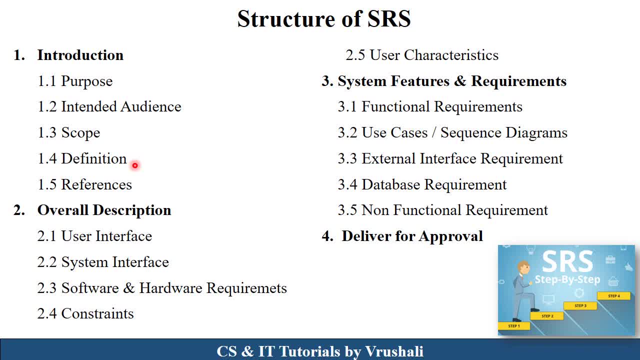 there is a hod. some user can't understand what is hod. so hod means head of department. so everything, every definition have mentioned clearly. the last one is the references. references means project head, check that whether the particular application is already developed or not. if it is already developed, refer those particular application and also add some new features in it. 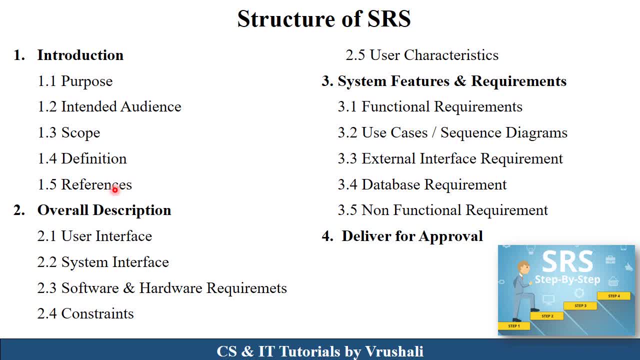 so this, all information have entered into the references. now second part of srs document is overall description. the first one is a user interface: means every user having the different interface, student having another interface, teacher having another interface, same hod having another interface. so every user having different interface, different features. next one is a system interface. 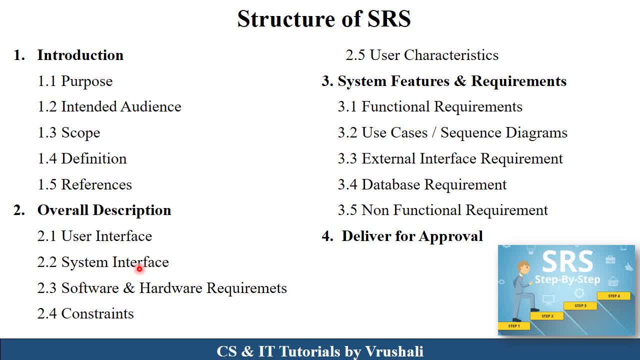 system interface means which type of server used, for example apache, http, http, ps. so this all information have mentioned here. next one is the software and hardware requirements: which type of software, which type of programming languages and framework used for development purpose, and hardware requirements for accessing a particular college management system application. 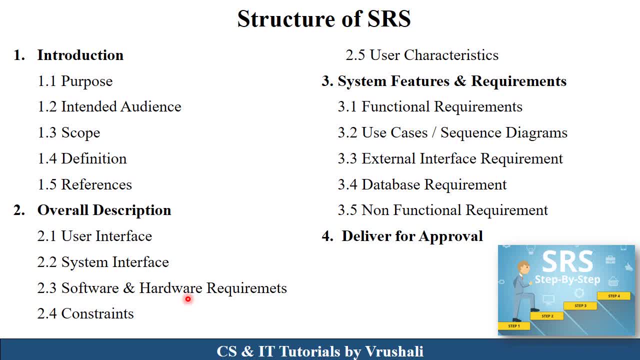 which type of hardware used, for example keyboard mouse, then monitor. so this all requirement list mentioned here. the last one is a constraints. constraints means condition. for example, students can't edit their attendance or can't edit their marks, right, this is a condition. next condition is you can enter a password while login only three times. after that it display the error. 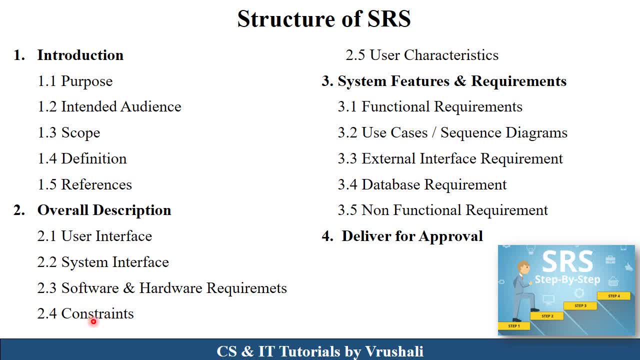 error of fail. so this type of conditions have mentioned under the constraints. and next one is a user characteristics. user characteristics means interface of every user, means teacher, having mentioned the attendance of every student, student can't edit their attendance. teacher also set the question paper by using the particular 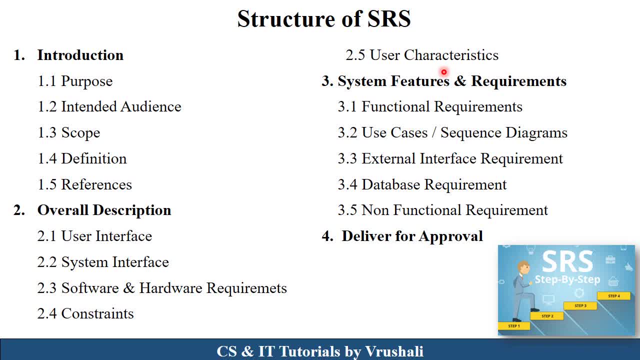 application and user can't edit their question paper. user just mention their answers, right? so these are the user characteristics. develop a project as per the user features. the next part is system feature and requirement. here you have to mention all the functional. requirement means which type of features customer want. use case and sequence diagram. it display how your product. 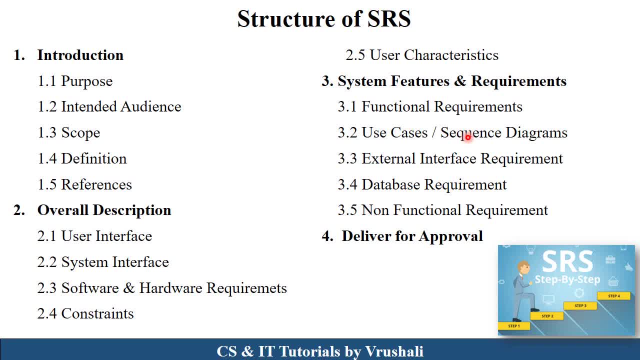 is looking in future. for example, first there is a registration form. use a, register your system. after that there is a username password. after clicking on login button, next page is open. so the view means after clicking on button, which page will be open. so their sequence. so these all things are showing by using a particular diagram. 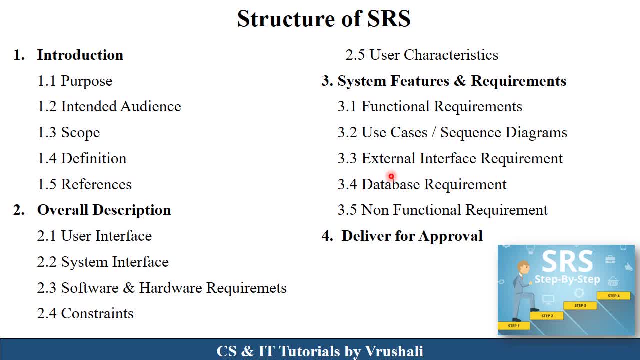 next one is the external interface requirement. for example, a particular student want to pay up their fee, college fee- okay, when they click on pay button, it redirect on the google pay application or phone pay application. means they use external app, external interface. so this all information have mentioned. 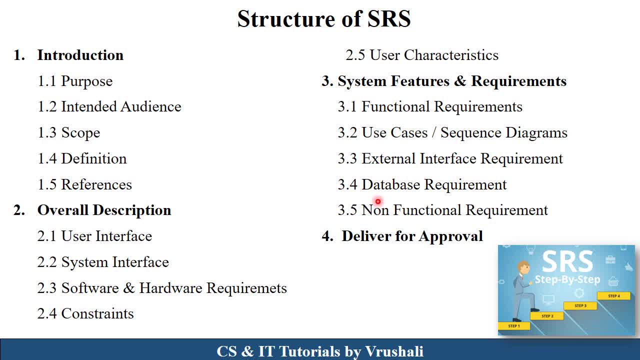 here. the next one is a database requirement. which type of database used for development purpose, like mysql, oracle, etc. then non-functional requirement means all the requirement related to the performance, their security, their cost. then their portability means a particular product work on windows operating system as well as linux operating system. this is called 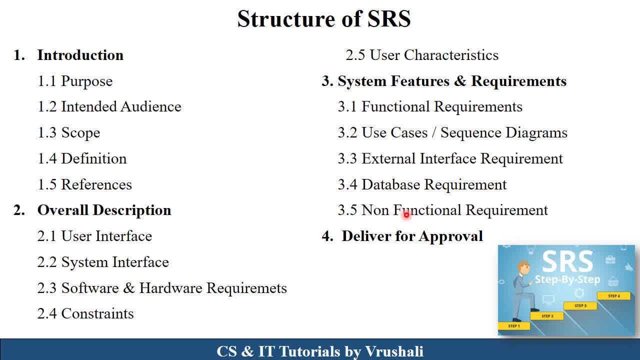 as portability, then their accuracy quality. so this all requirement mentioned under the non-functional requirement. and last one is a deliver for approval means this all srs document. after completing deliver to the customer. customer check all this document. if customer want any changes, they do all this changes under this document. if customer satisfy, then 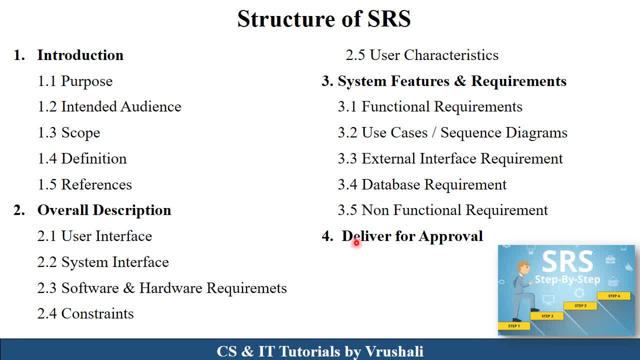 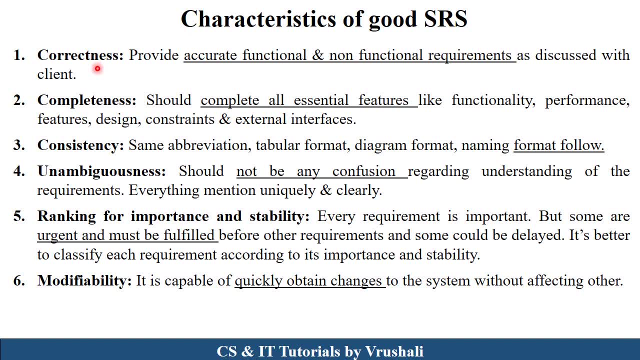 this document sent to the next designer or developer development team. so this is all about structure of srs. the next one is a characteristics of good srs. so while writing srs, the first one is their correctness means each and every functional and non-functional requirement discussed with customer mentioned accurately. 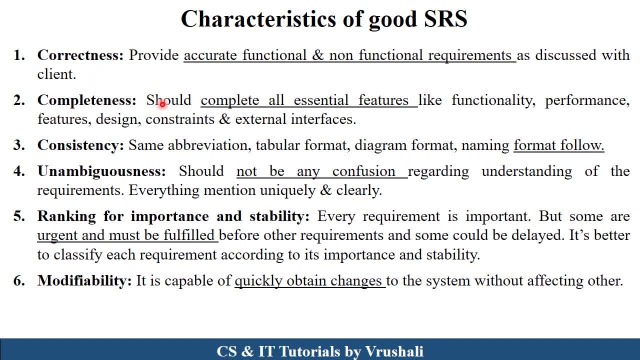 correctly: completeness. completeness means it should mention all the essential features like their functionality, performance. which type of design constraints customer want everything mentioned clearly or completely consistency. consistency means complete. srs report follow a particular format, the format related to the tables diagrams. so they follow a particular format here: consistent format. next one is: 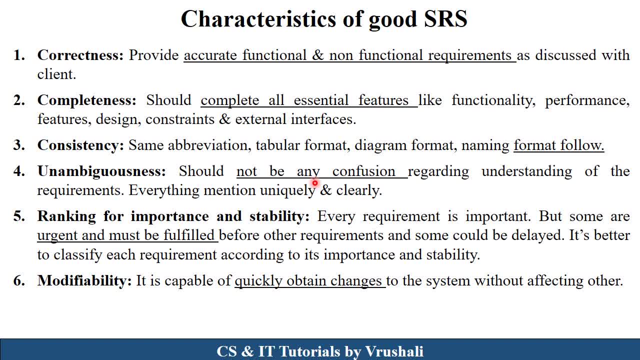 an unambiguous. unambiguous means they should not mention any confusion between a customer and developer: everything mentioned uniquely and clearly. next one is a ranking for importance and stability. it means suppose there are total ten requirements from that, ten requirements customer want on urgent basis. so the srs document, mention which type of requirements are. 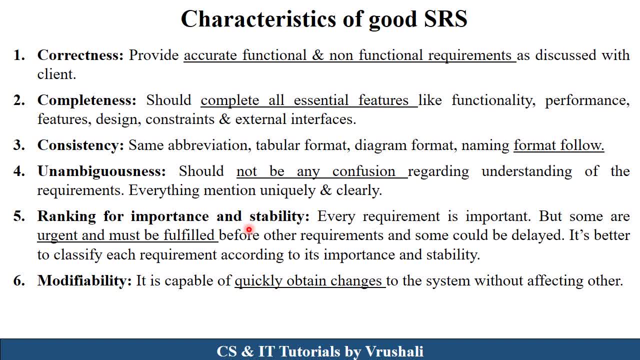 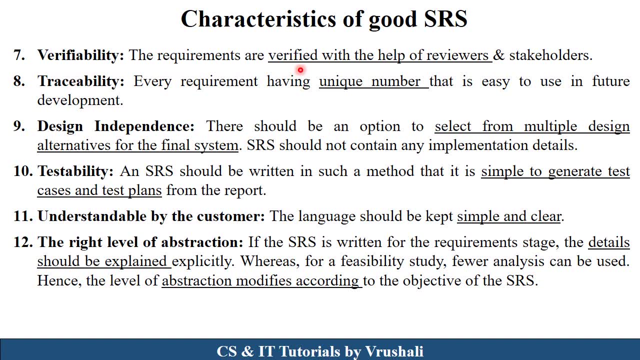 on urgent basis and which type of requirements are not urgent basis? next one is a modifiability. modifiability means if customer want any changes, it quickly obtain changes in particular system. next next one is a verifiability: means all the srs document, srs requirement is verified.